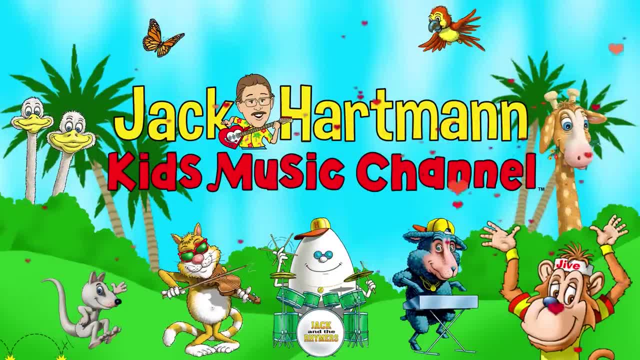 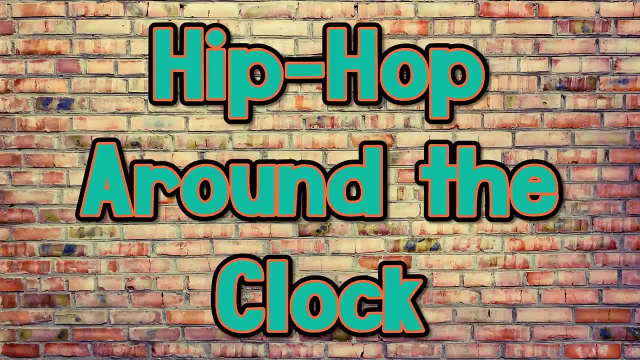 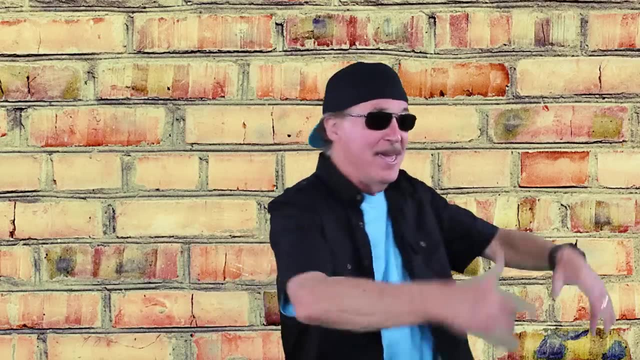 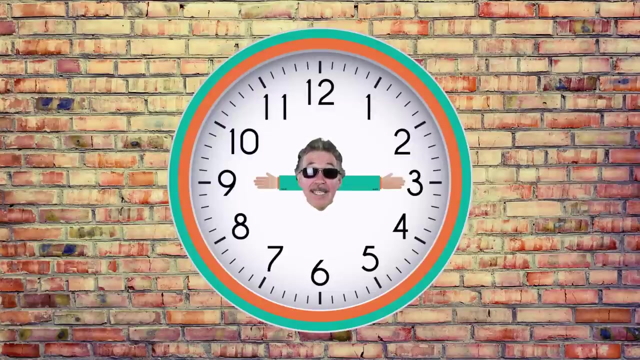 Jack Cartman Kids in the Channel Hip Hop around the clock, Hip Hop around the clock. When I say the time, you stop. If you're at the time you say Hip Hop, Hip Hop. Then the time on the clock: Hip Hop around the clock, Hip Hop around the clock. 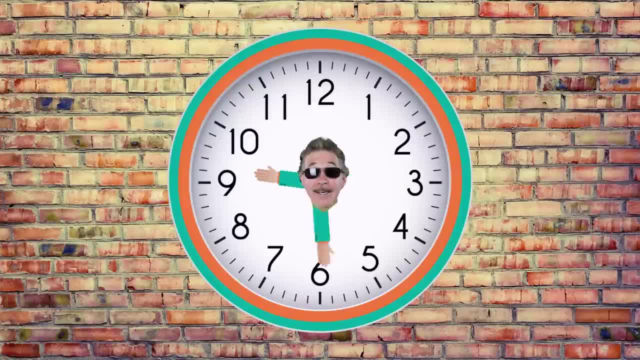 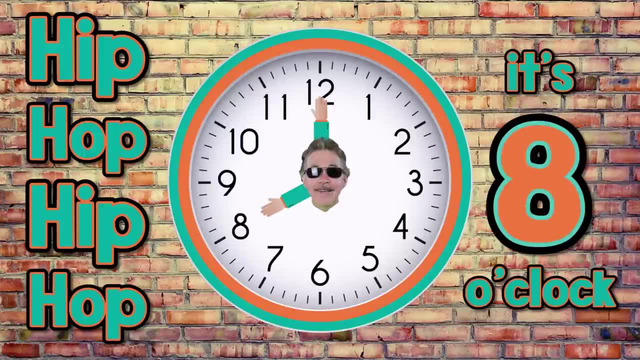 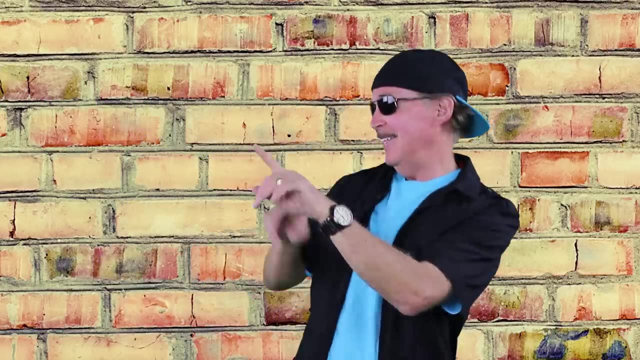 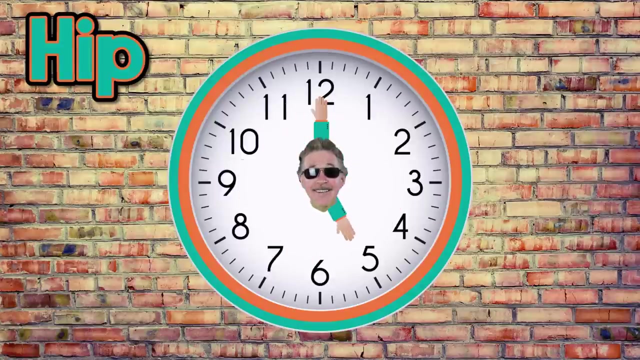 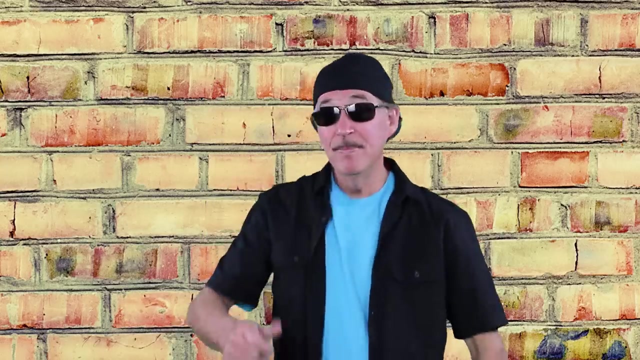 Now the time is eight o'clock. Hip Hop, Hip Hop. It's eight o'clock. Hip Hop around the clock. Hip Hop around the clock. Now the time is five o'clock, It's five o'clock. Hip hop, hip hop. It's five o'clock. Hip hop Around the clock. 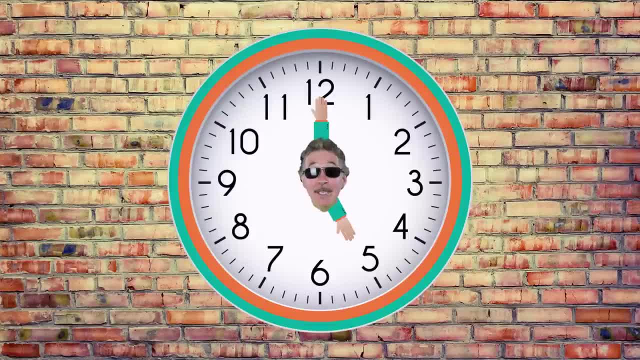 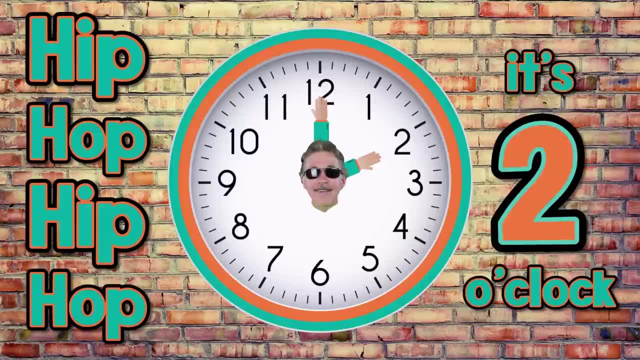 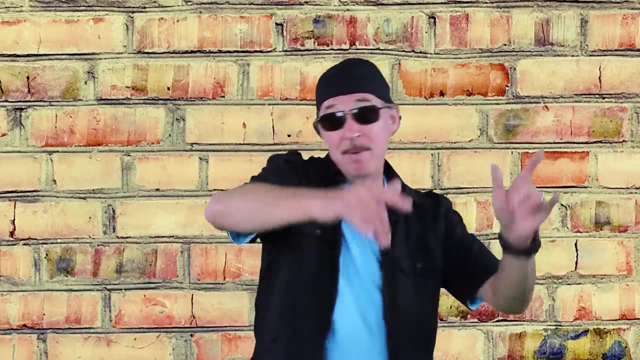 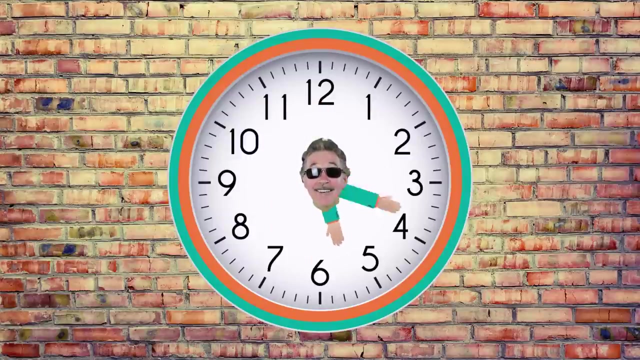 Hip hop Around the clock. Now the time is two o'clock. Hip hop, hip hop. It's two o'clock. Hip hop, Hip hop Around the clock. Hip hop Around the clock. Now the time is eleven o'clock. Hip hop, hip hop. It's eleven o'clock. 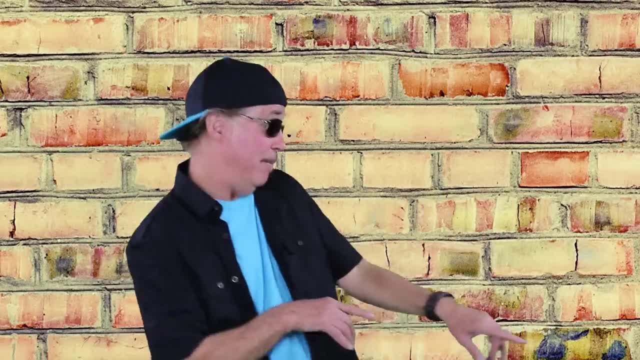 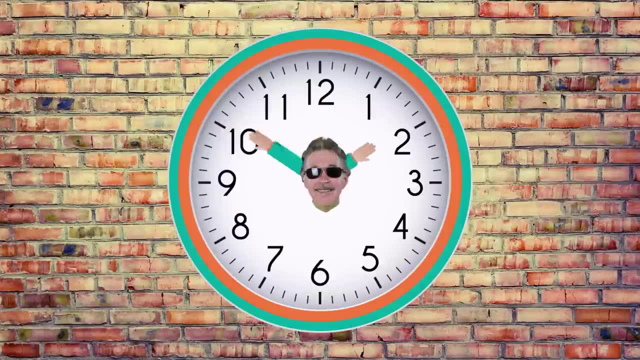 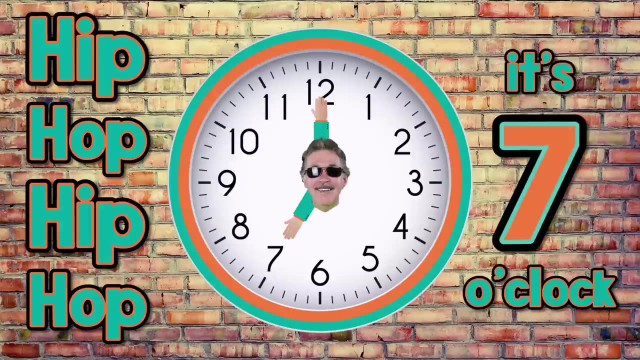 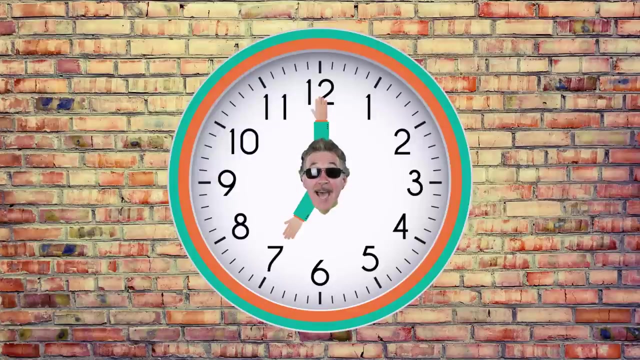 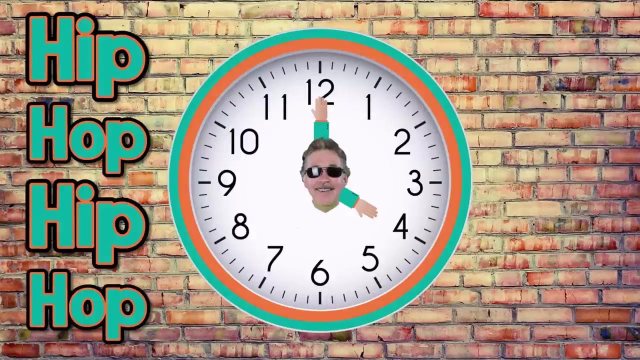 Hip hop Around the clock. Hip hop Around the clock. Now the time is seven o'clock. Hip-hop, hip-hop. it's seven o'clock. Hip-hop around the clock. Hip-hop around the clock. Now the time is four o'clock. Hip-hop, hip-hop, it's four o'clock. 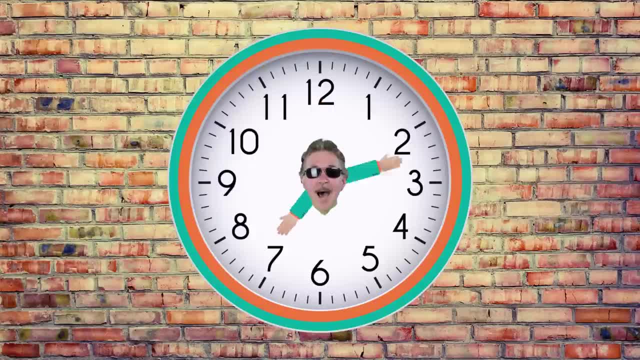 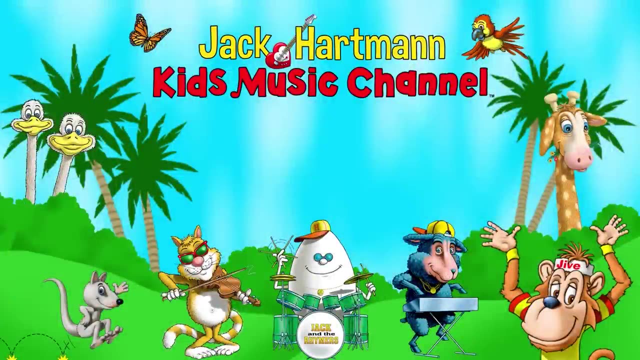